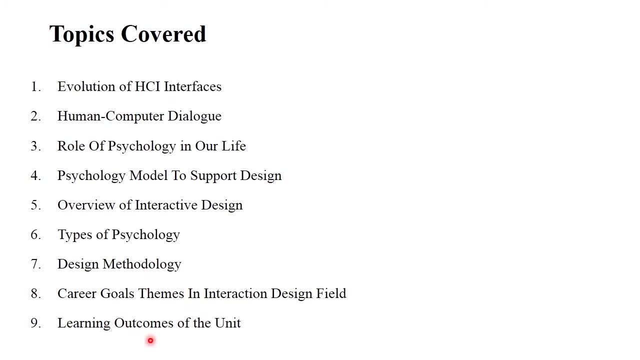 Career Goals, Themes in Interaction, Design Field and Learning, Outcomes of the Unit. These all topics are covered in this video. Or we can say this is the short approach or summary of 2nd Unit, That is, Understanding the Human Clear. 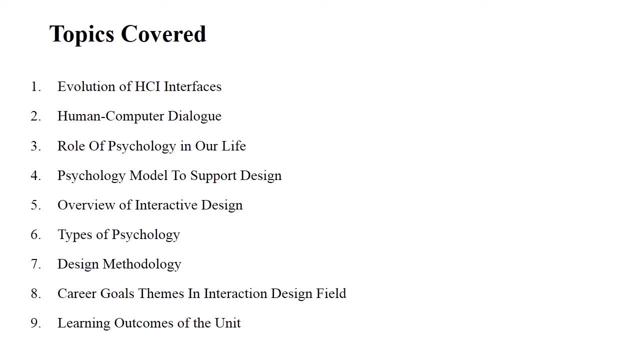 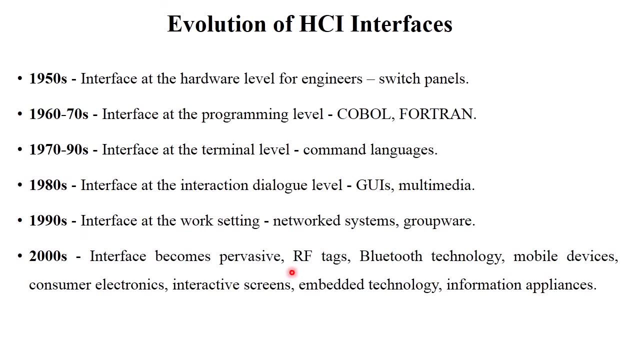 Ok, So let's see one by one, That is Evaluation of Human-Computer Interaction Interfaces. Next Now see here: This is Generation or Hierarchical Structure-Wise: Generation or Evaluation of Human-Computer Interaction Interfaces, How Human-Computer Interaction or different types of latest technologies are involved in this era. 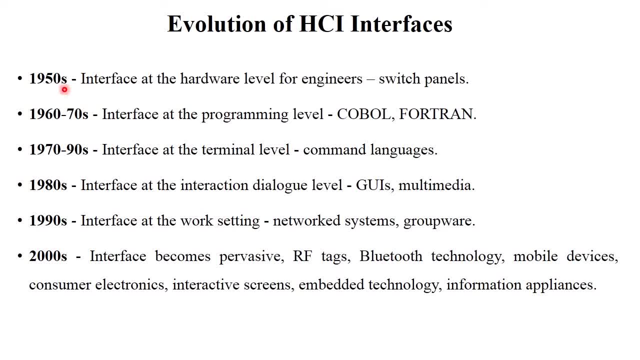 So we started from 1950s. In 1950s there was interfaces at the hardware level for engineers and switches. Right Then, in between 1960-1970,, there was COBOL and Fortin. This kind of languages are developed. 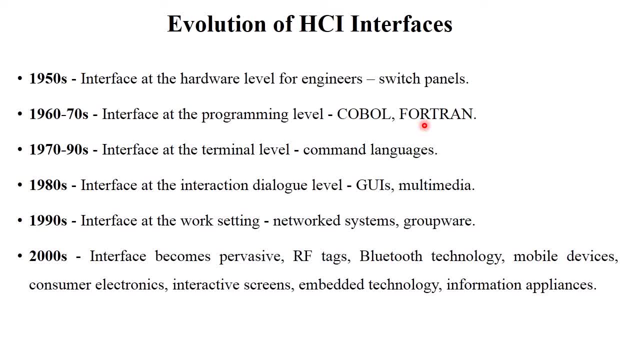 Ok, COBOL and Fortin is earliest language, Means in before C or C++. this COBOL and Fortin, These languages were developed. Ok, Then in between 1970-1990, command languages were developed. 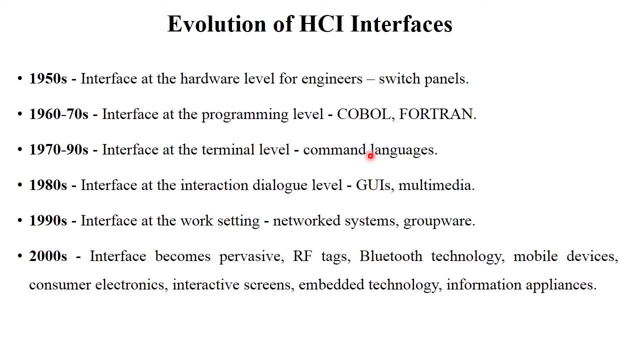 Ok, We all are familiar with command languages, Different types of commands here, Different types of commands used in Linux, Unix, etc. Ok, Now in 1980.. 1980s, interfaces at the interaction dialogue level. Interaction dialogue level means different types of multimedia, televisions or graphical user interfaces. 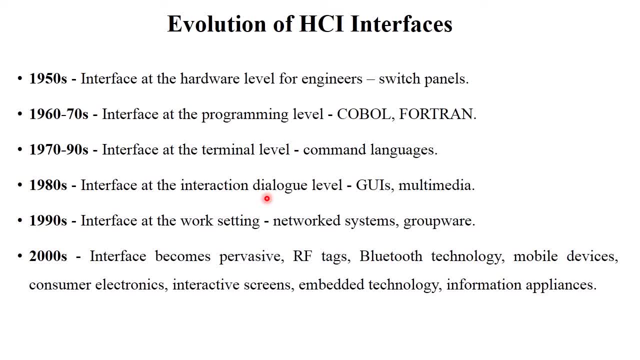 This kind of products were developed in 1980s era. Ok, Now next 1990s. In 1990s there was Networked System or Groupware. This kind of products are developed. Ok, This kind of products was developed. 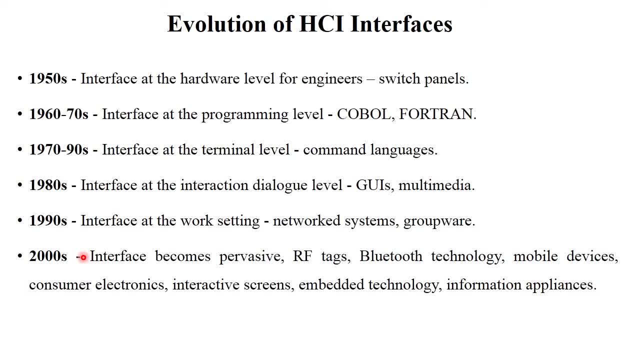 Ok, Now in 2000.. After 2000, we are familiar with, after 2000 all the products Like interface becomes RF tags, That is, waves, radiofrequent waves, Bluetooth technology, mobile devices, consumer electronics, interactive screen, embedded technology and information appliances. 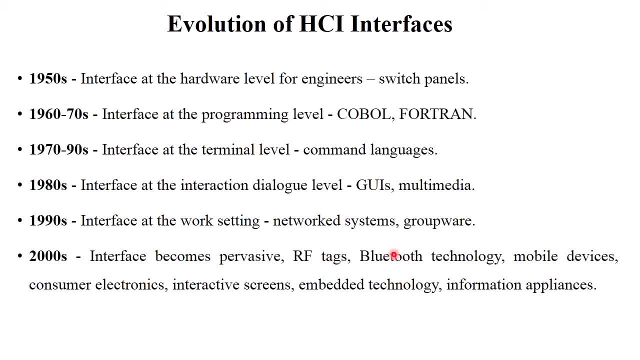 Right, We all are familiar with this: all types of languages products, Right Languages products, then multimedia, etc. Ok, So this is the evaluation of human-computer interaction Means humans are interacted with the computer through all these types of products in each and every era or each and every year. 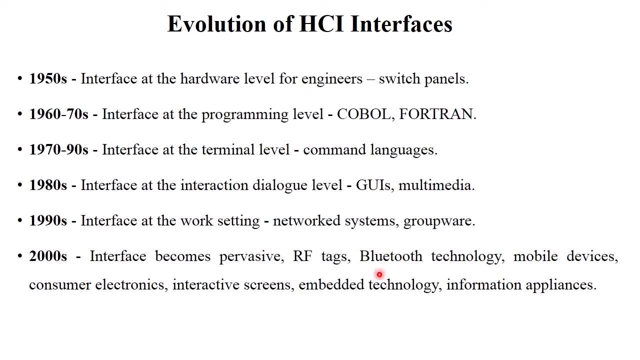 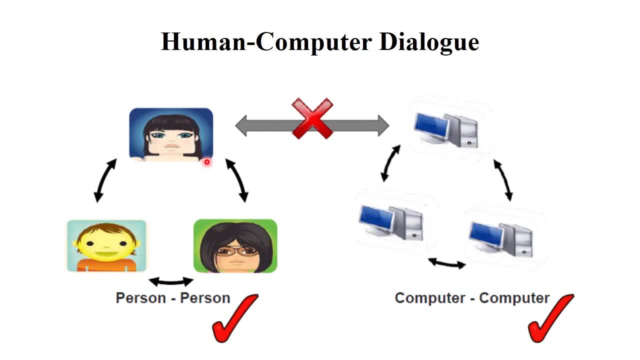 Right, So this is the evaluation of human-computer interaction. Ok. Next, Human-computer dialogue: See in this diagram, Or what do you understand by this diagram? See, there are total persons and this is computer. Ok, So human-computer interaction is not a person to computer connection. 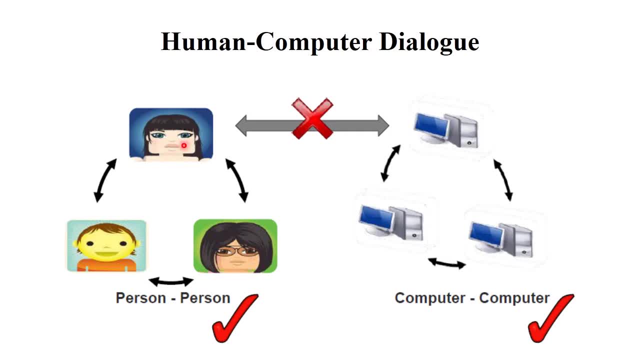 Ok, Human-computer is there are different groups of persons, is connected or is communicated with different groups of computers. Ok, So human-computer dialogue is the communication between group of persons to group of computers, Not a single one, Ok. 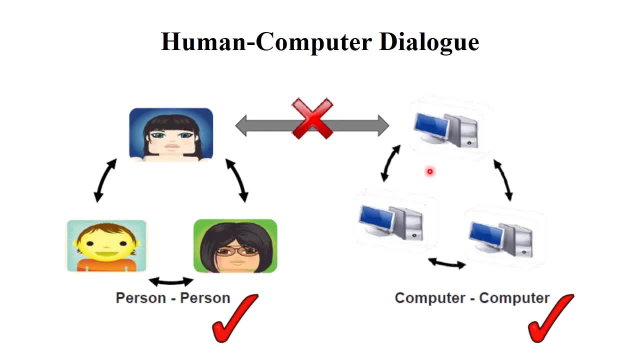 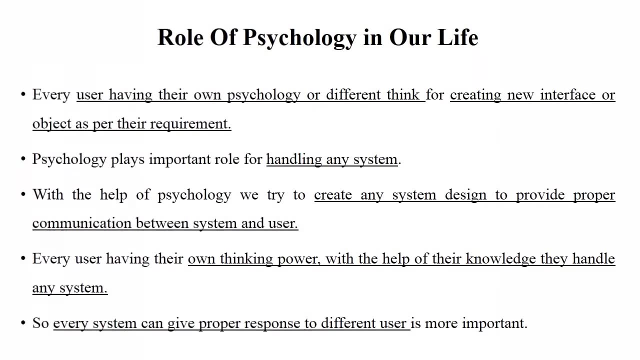 Not a single one is not occur here. There is many, to many connections in that Clear. So this is called as human-computer dialogue, Ok, Next. So now see role of psychology in our life And what is mean by psychology. 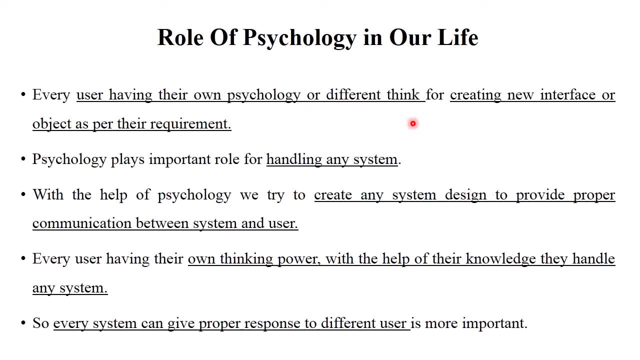 Users having their own psychology or different things for creating new interface or new objects, as per the requirement Right? I already told you there are different peoples. They have different ideas, Different skills, Different technical knowledges, Different thinking or different ideas. 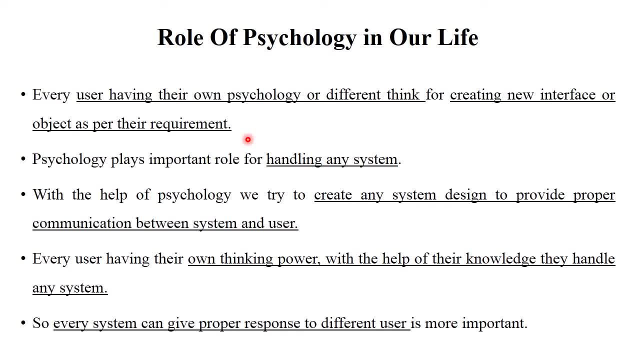 Ok, So this is called as psychology. Psychology of each and every persons are different, Clear. So this is the meaning of psychology. Psychology plays important role for handling any system or different systems. With the help of psychology, it create any system design to provide a proper communication between system and user. 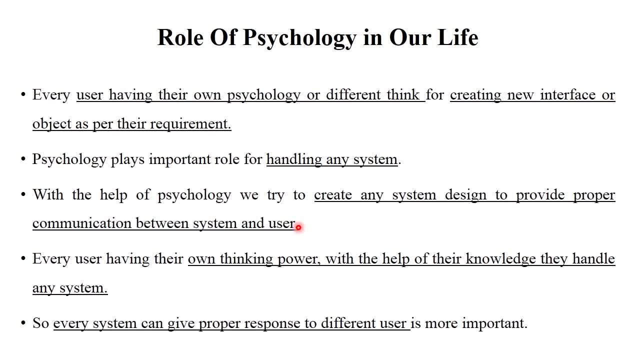 Ok, We know that Computers, Laptops, Mobiles, This kind of gadgets are developed by human Right. So this is the psychology of human. They generate or develop this kind of product and get more familiar with this By completing your daily work or daily task. 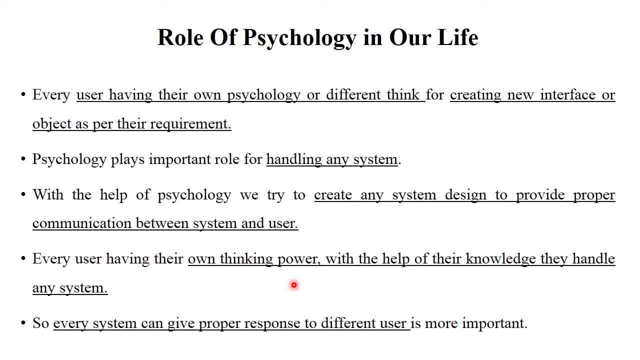 Right. So every user having their own thinking power. With the help of their knowledge, they handle any system. Every system can give proper response to different user. It's more important, Right, We can use browsers for searching purpose. We used multimedia. 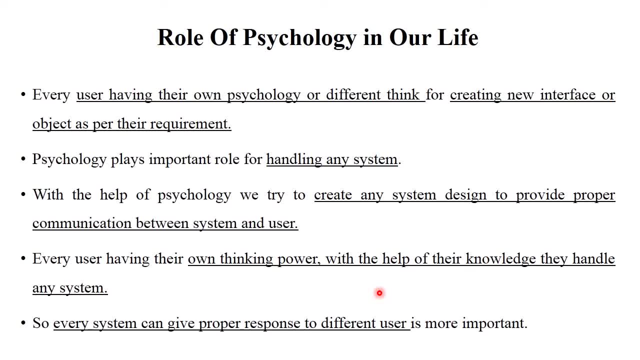 Right For enjoying purpose. Then we use different types of applications- Social applications, Financial applications, Right- So response of the system is different for each and every applications: Clear. So this is called as psychology or role of psychology in our life. 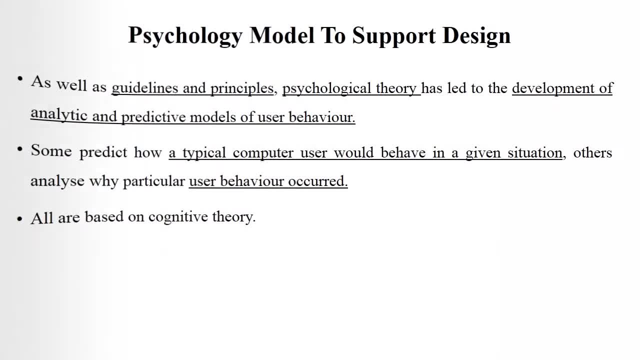 Clear. Ok. Next Psychology model that support design: Ok, So see, here There are different types of psychologies related to the guidelines and principles. There are different types of psychological theories for development of new products. Ok, So they require different types of guidelines and principles. 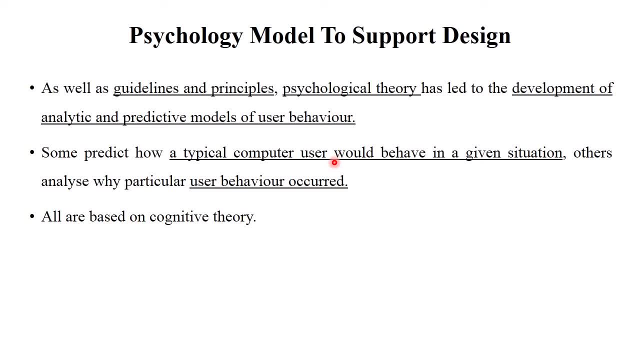 And you must follow that. guidelines or principles for developing the product: Ok. So development of analytics and predictive models of the user behavior: Ok, I already told in my previous video That is user centered design. Ok, To make the particular product as per the requirement of the customer. 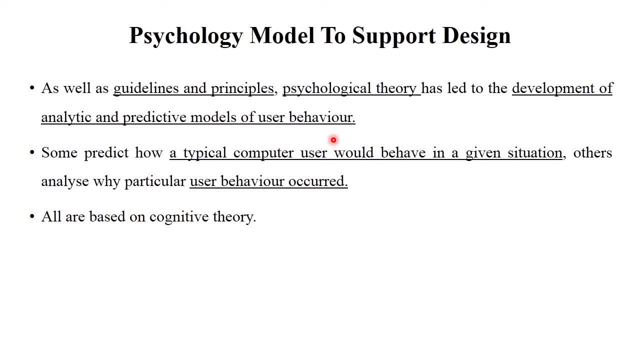 You need to involve customers for each and every phases of that software development life cycle Clear. So this is called as psychology model that support the design. Some predict how a typical computer users would behave in a given situation And others why particular user behavior occurred. 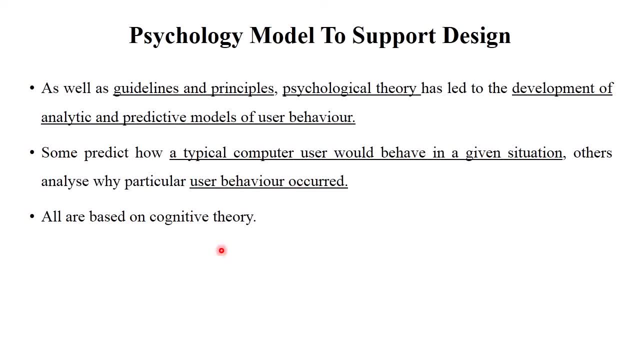 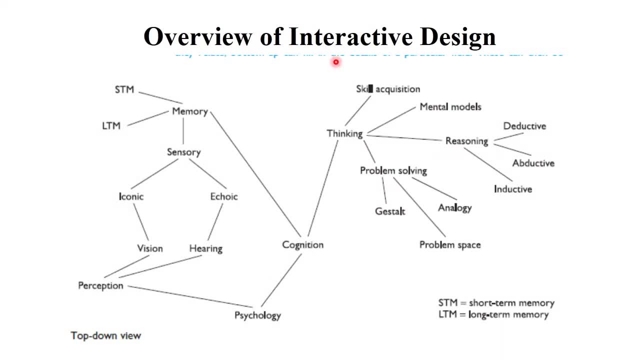 Ok, So all are based on cognitive theory, Clear. So this is the psychology model. Next See here. This is overview. interactive design: We already learnt memory thinking in my previous videos. Ok, So see here: Memory. 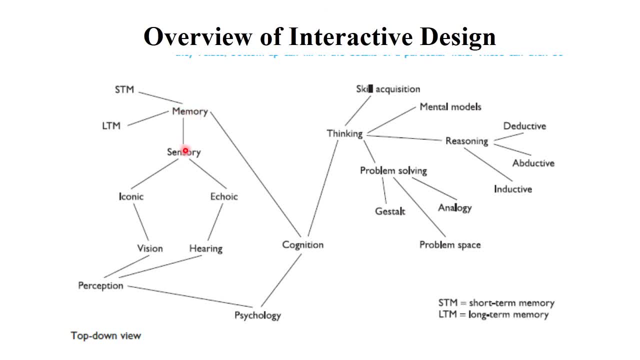 Memory has three types: Sensory memory, long term memory, short term memory. Right Sensory again has two types: Iconic, echoic and one again haptic memory. Ok, So this is the psychology model Next- So this is the overview- interactive design. 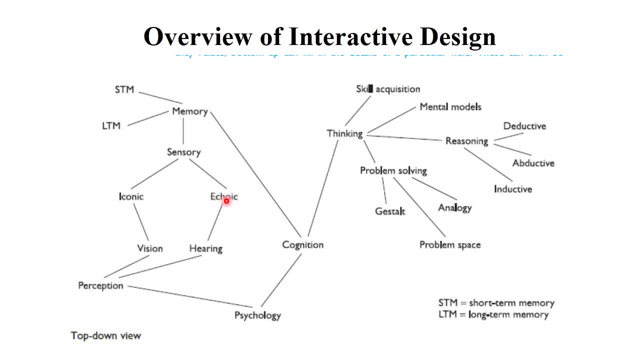 We already learnt memory thinking in my previous videos, Ok. So see here Memory Meaning. one again: haptic memory, Ok. Iconic means vision or perceptions. Echoic memory means hearing or audible memory. Clear Now another way. there is thinking. 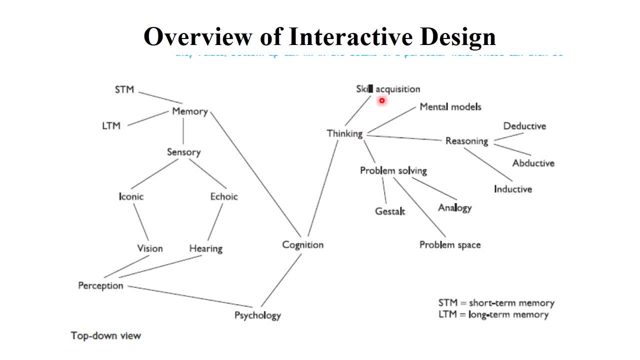 Thinking includes skill acquisition, mental models and reasoning- Ok. Reasoning also has three types: Deductive reasoning, adductive reasoning and inductive reasoning- Ok. Problem solving approach includes gestural theory, problem space and analogy. Ok, So this is the psychology model. 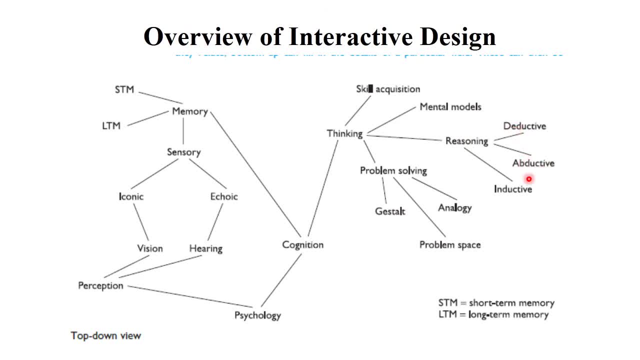 Next: See here: See here. So this is the psychology model. Ok, So this is the psychology model. Ok, So this is the psychology model. Next, So this is the psychology model and analogy right. so each and every points regarding memory, thinking and other theories. 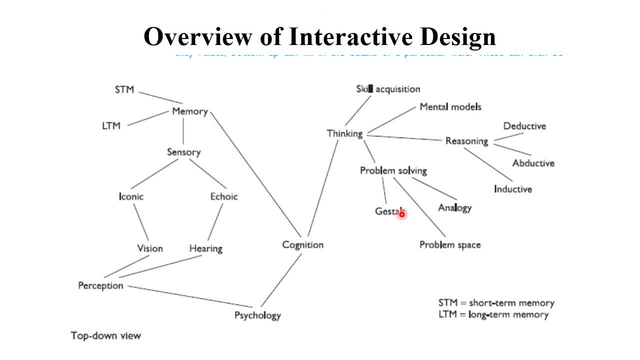 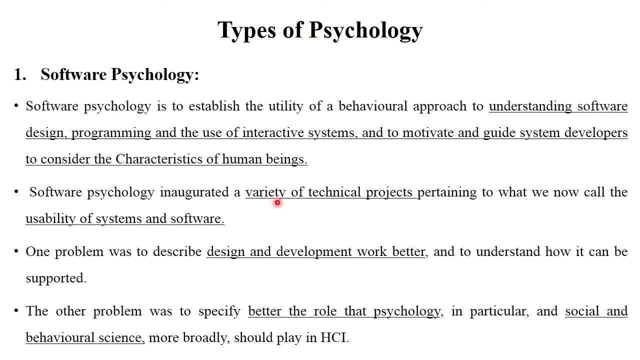 we discuss or will learn in my previous videos. hope so you understand it and you are familiar with this point. okay, so this is complete overview of interactive design, clear, okay. next, types of psychology: okay, so this point is not included in your syllabus, but, uh, this is general points. we are, we all are familiar with this. okay, so there are actually two. 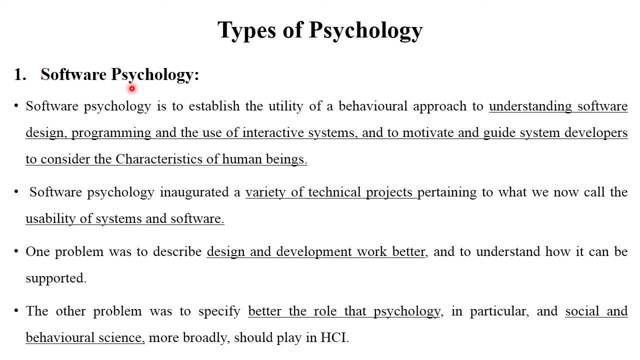 types of psychology, that is, software psychology and cognitive psychology. okay, so let's see one by one. the first type of psychology is software psychology. what is mean by software psychology? so software psychology means to understanding the software design, programming and the use of interactive system. it motivate and guide the system developers to consider the characteristics. 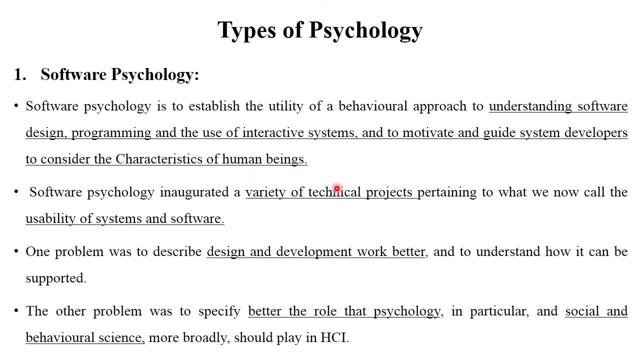 of human beings, right. see, for example: uh, when you used your mobile, you know that. how to use mobile, which types of applications are open, okay, how to use that uh audible, or how to use video calls, etc. so this is called a software psychology: users are familiar with that particular product, clear. so this is 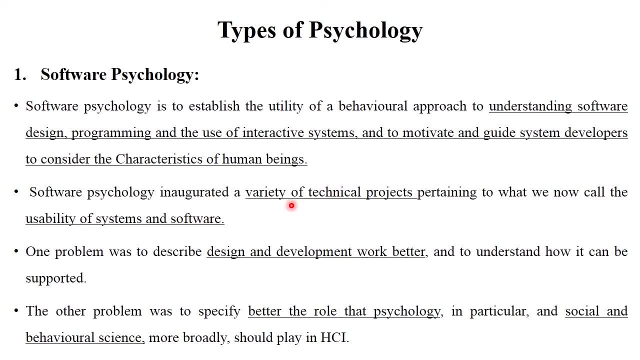 called a software psychology. so software psychology also includes variety of technical projects. okay. it makes the usability of system and software okay. so usability means easy to use and easy to learn. you always develop a particular product it's very easy to use, easy to learn, which is usable by each and every people. 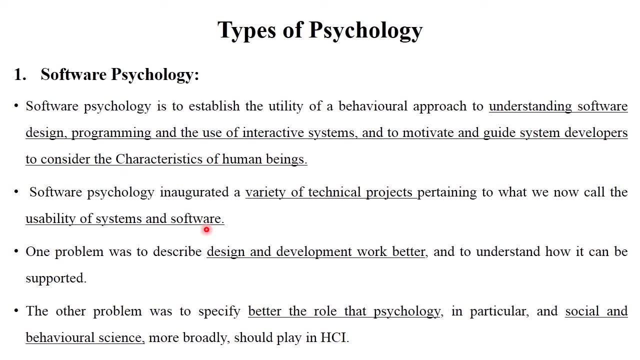 either technical or non-technical people clear. so software, psychology, design and development work better. it makes the work more better in nowadays, right? so the other problem was to specify better the role that psychology, a particular and social and behavioral science, human, computer interaction is kind of part. they work each and. 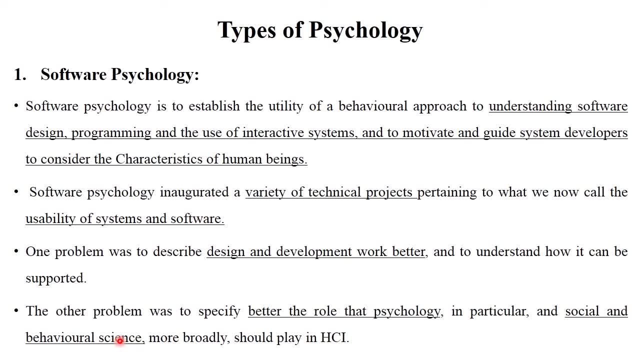 every field, whether it is social field or behavioral science field. okay, we already uh learn about multidisciplinary fields in human computer interaction in my previous video. clear, so this is called a software psychology. okay, so simply, software psychology means how user use that particular product. clear, so this is called a software psychology. okay, so, simply software psychology means how user use that particular product. clear, so this is called a software psychology. so this meaning of formative companies, or 밖에 Houston Electronics software psychology means coherιο software helps a user to understand these types of interactions. other topics is body shape, then how the twoa use specific industry. space rupees 투. 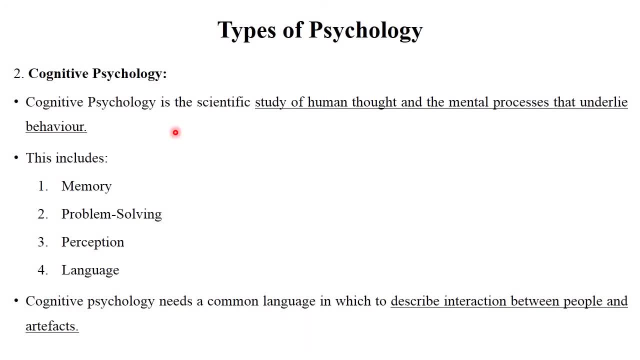 psychology. okay next, so second type of psychology is cognitive psychology. what is meant by cognitive? cognitive means study of human thought and mental process that underlie behavior. okay, so cognitive simply means study of human and their mental process. okay see, psychology has two types: softer psychology and cognitive psychology. softer psychology means study of human towards the 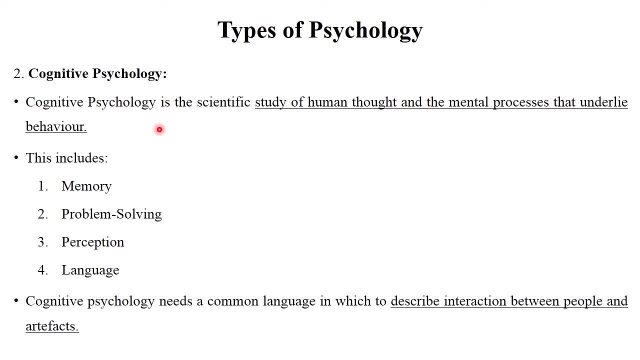 software means how to use that particular product- okay. and cognitive psychology means study of human and their mental process, which not includes any software- okay. so cognitive psychology includes memory problem-solving approach of the user perceptions and languages- clear. so cognitive psychology need a common language in which describe the interaction between people and 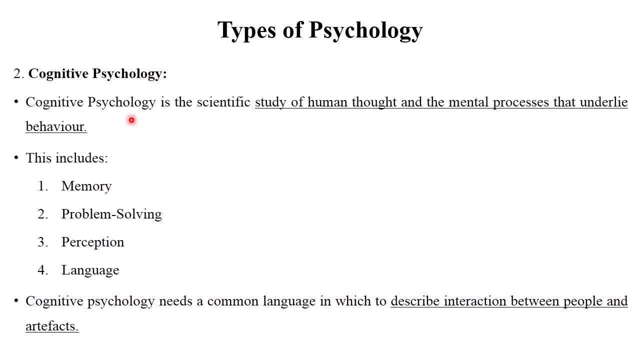 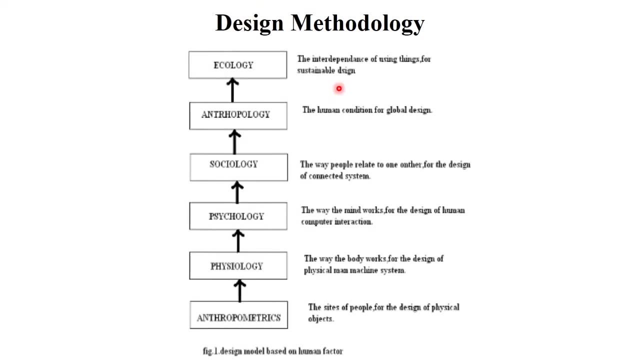 artifacts. clear. so this is called as cognitive psychology. it study the human behavior, human memory, human languages and human problem-solving approaches, etc. clear, okay. next now design methodology. okay, there are different types of designs, like ecology, anthropology. okay, what is meant by ecology? ecology means interdependence of using things. 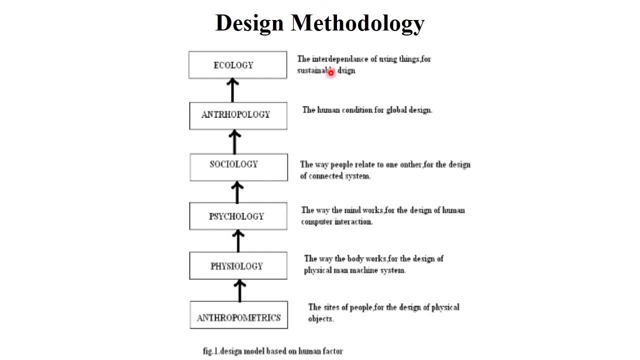 for sustainable design. okay, means make different approaches of design. and then anthropology means human conditions for global designs. okay, now sociology. sociology is a study of people, how to relate one another for the design of connected system. then psychology- psychology- study of mind, work of the design of human computer interaction. then physiology is the study of body. 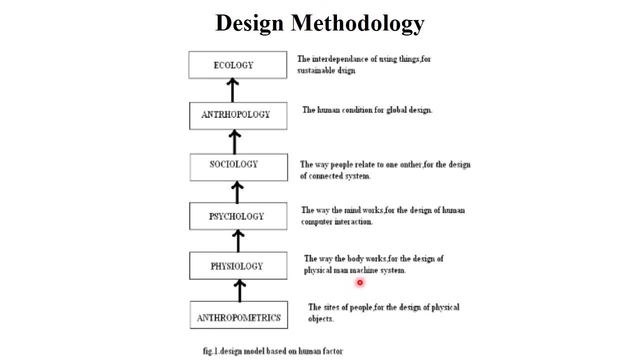 work how to design of physical man machine system. and anthropometrics means it is a study of sight of our body. so this is the design of methodology. in this way, overall, human computer interactions are work clear. okay, next career goals, themes in interaction design field? okay, see human computer. 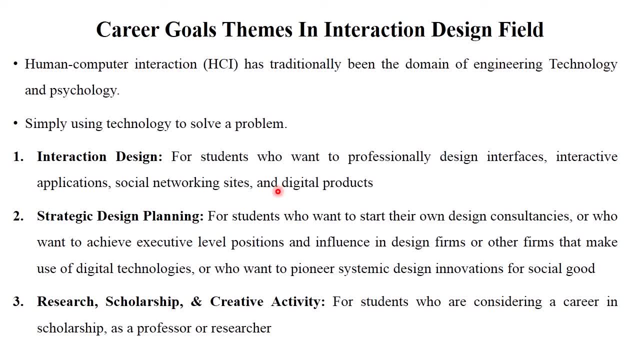 interaction. this field also provide different types of Career approaches. okay, you should also career in this field. so human computer interaction has traditionally been domain of engineering, Technology and psychology: simply using technology to solve the problems. okay, See, here there are different career goals. The first one is interaction design. 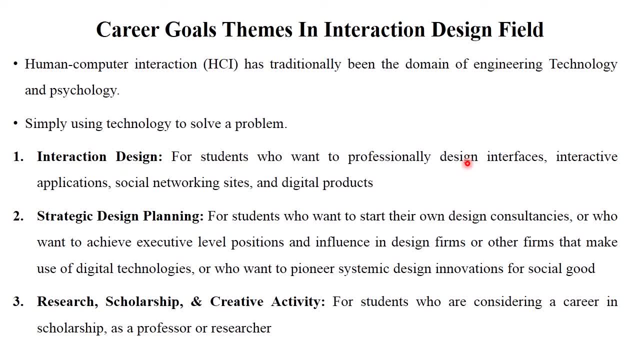 Okay For the student who want to professionally design interface, or we can say design engineers, interactive applications or make social networking sites and digital products. Okay, So interaction design is also field of human computer interaction. You should make your career in this field. 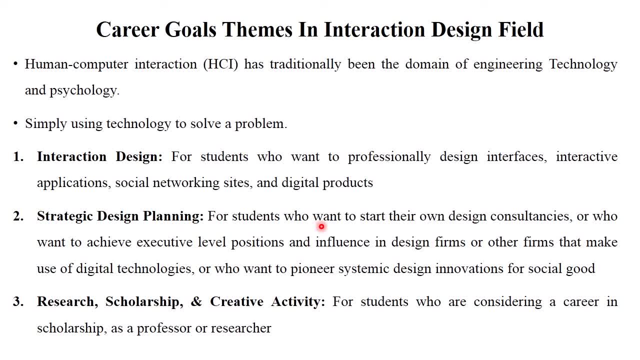 Then a strategic design planning For the student who want to start their own design consultancy, Who want to achieve execution executive level positions or influences in design firms, Right Or digital technologies, And also who want to pioneer systematic design innovations for social goods. 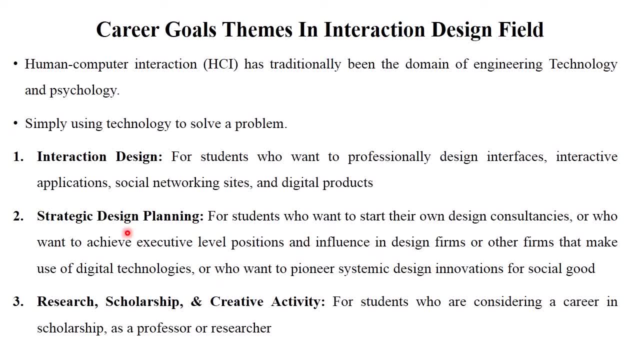 Okay, So this kind of opportunities also available in human computer interaction field. And the last one is research, scholarship and creative activity. For the students who are considering a career in scholarships, as well as professors or researchers. Okay, They have also different opportunities in this field. 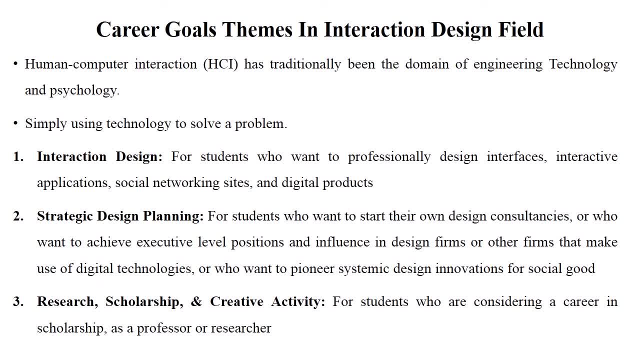 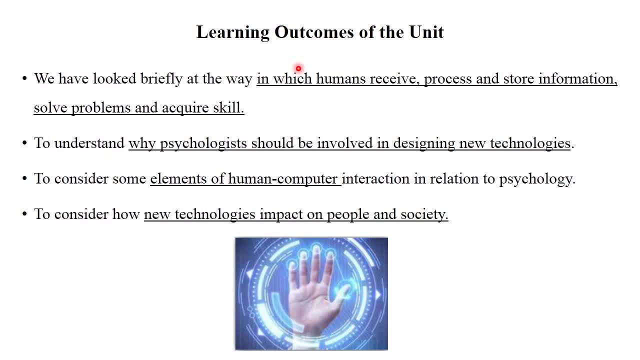 Okay. So see, these are the career goals. You should go through this and also make your career more successful. Clear, Okay. Next Outcome of this second unit: Okay, We have looked briefly in the way We also learn in second unit. that is human, how human receive different types of memories. 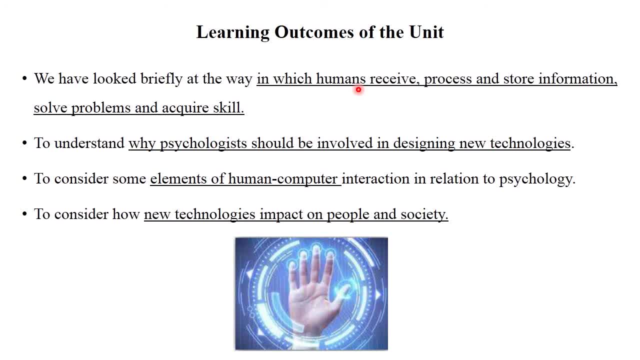 Input output channels. Then how to store the information: Okay, How to solve problem, Thinking and designing. Right To understand why psychologists should be involved in designing new technologies. Also consider some elements of human computer interaction And also consider how new technologies impact on people and also on society.